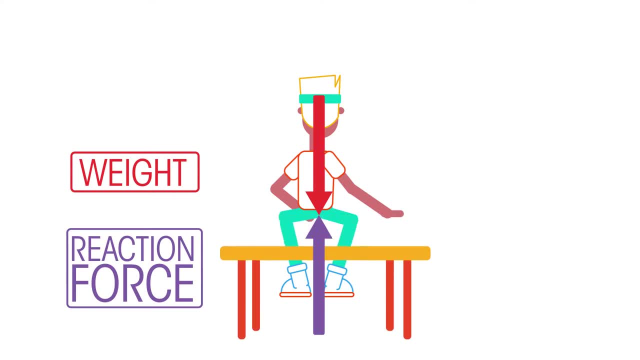 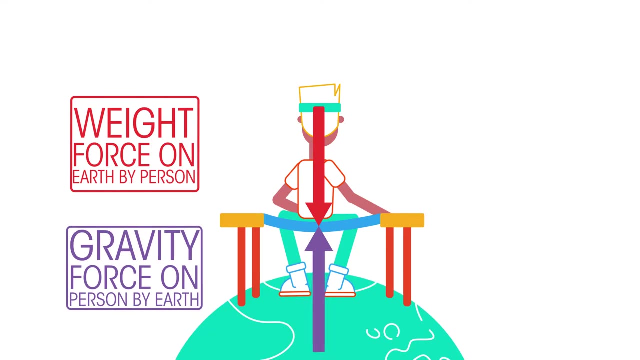 on the person. It's easier to see this reaction force if she sits on a trampoline instead. However, there are actually two pairs of forces acting here. The man's weight is balanced by the gravitational force he exerts on the Earth. He is prevented from falling towards. 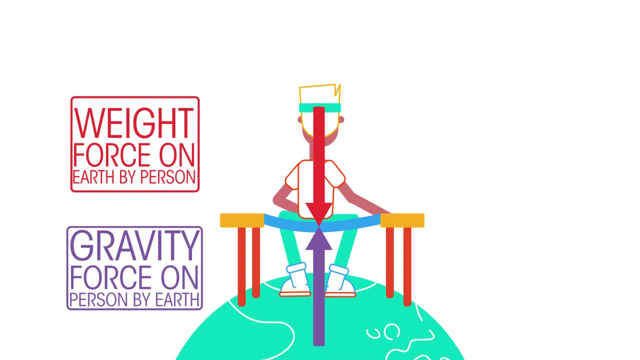 the Earth's centre because of the upward pressure of the force. The force is not as strong as the force of gravity on the person. The force of gravity is not as strong as the force on upward force from the trampoline or chair, which is balanced by the force he exerts on. 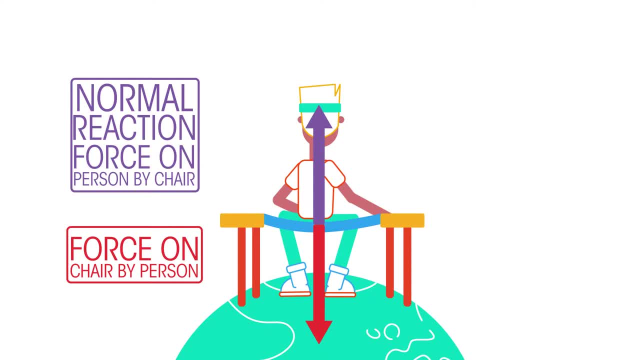 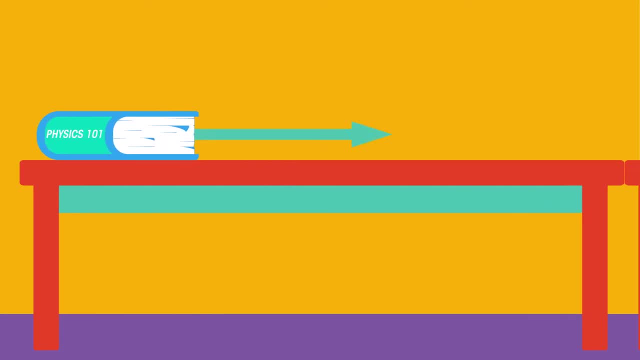 the chair. The forces are equal in magnitude or size, but opposite in direction. Or pushing a book at constant speed across a table: The force pushing the book acts towards the right. The force of friction opposes this and acts towards the left. 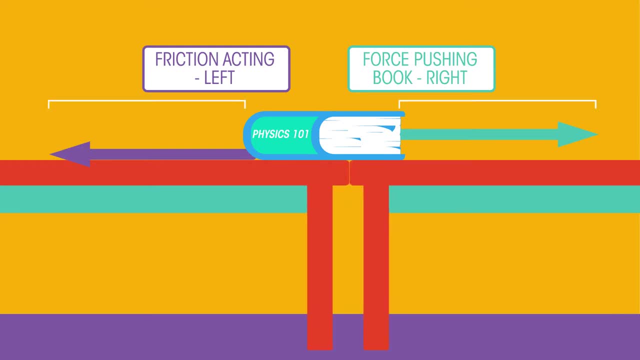 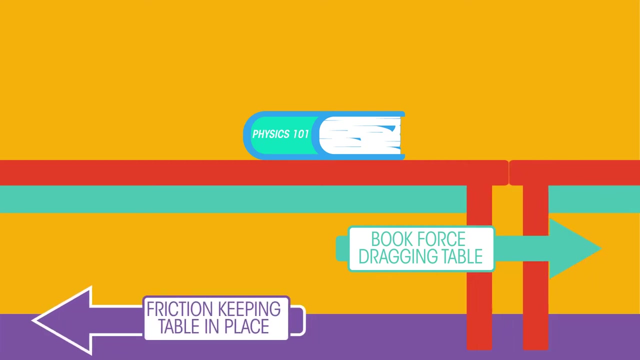 The arrow vectors are equal in length because the magnitude of these forces are equal. There is another pair of horizontal forces acting here. The book is trying to drag the table as it is moved to the right, But the table is kept in place due to the opposing 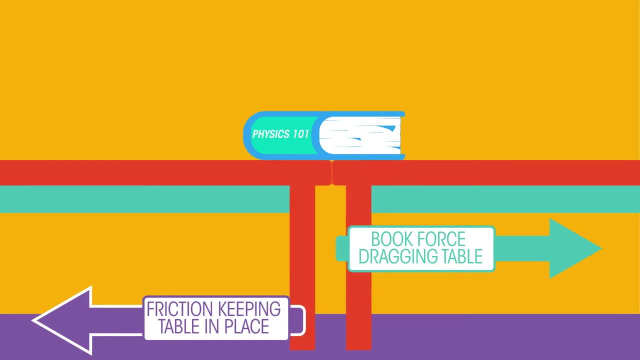 frictional force where the table legs touch the floor. We mustn't forget the pair of vertical forces acting here as well: The weight of the book on the table changes as the book moves to the right, The force applied to the table and the upward reaction force of the table on the book. 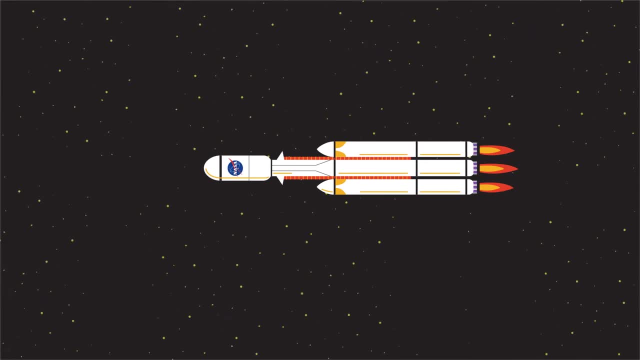 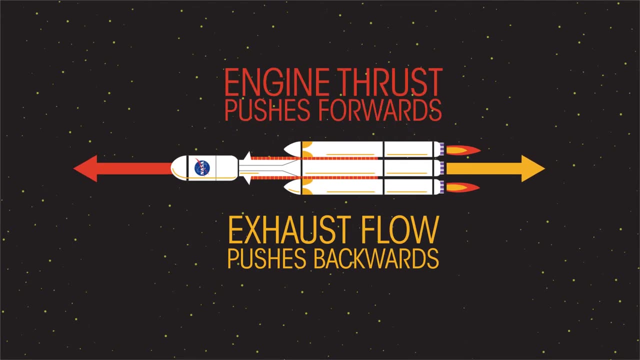 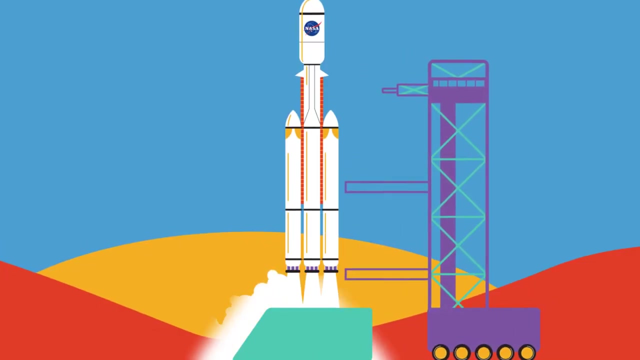 Consider a rocket engine in outer space. Hot gases are expelled from the back. The rocket pushes against the hot gases and the gases exert a force on the rocket which causes it to accelerate At liftoff. there is another pair of forces between the rocket and the Earth. 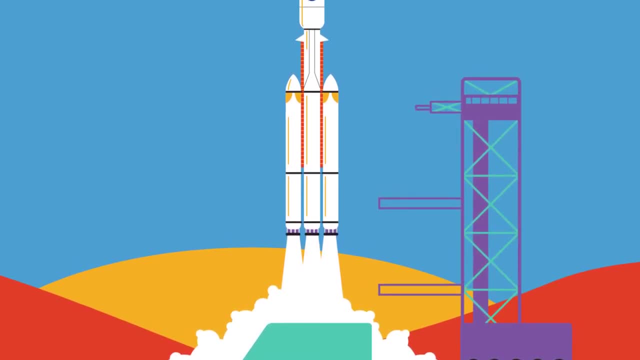 As we saw before, with the chair and the book. So there are now two forces on the rocket. If, as we hope, the force from the exhaust gases is greater than the force from the Earth, its weight, we will get liftoff.